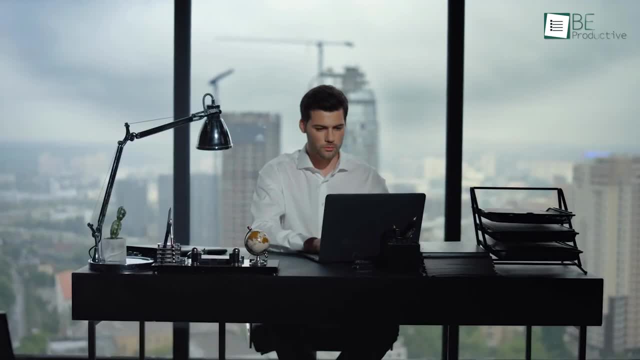 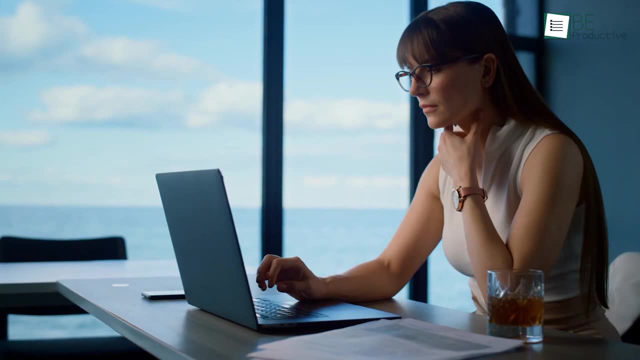 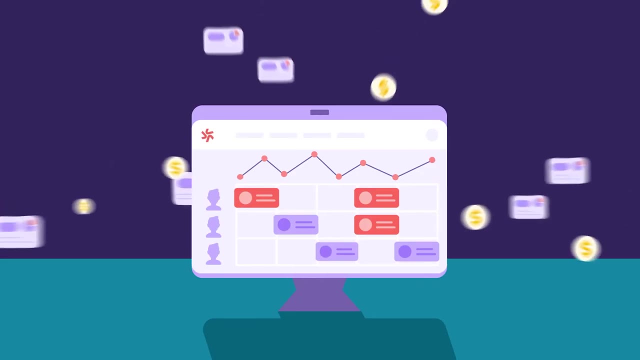 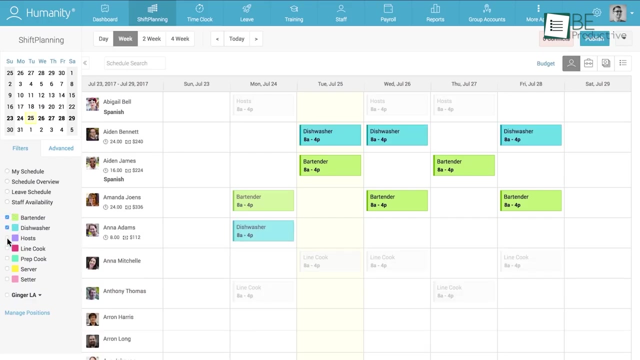 No matter how large or small your business is, creating a perfect schedule for your employees and notifying them manually is time-consuming and exhausting. To lessen that long, tedious process, many scheduling softwares are available. So, among those various options, we have come up with a list of the 5 intuitive employee scheduling softwares for you. 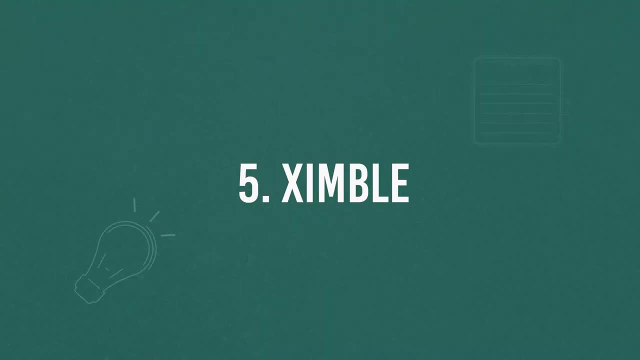 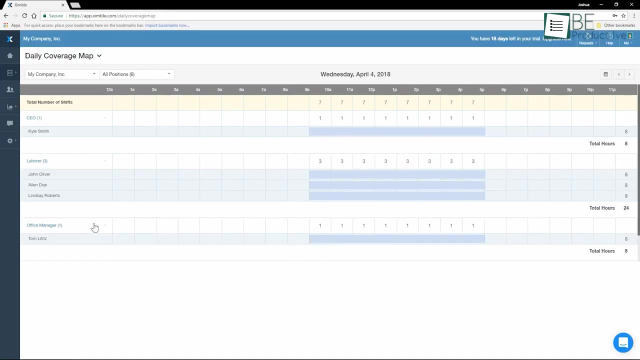 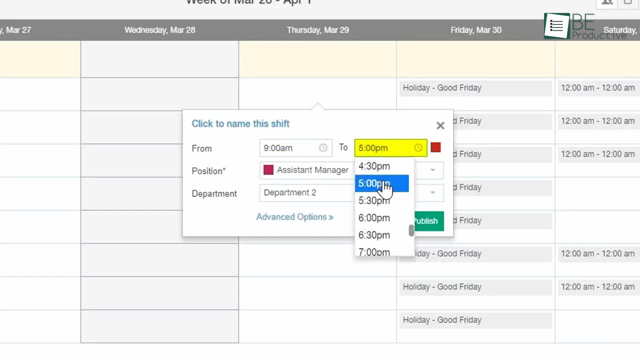 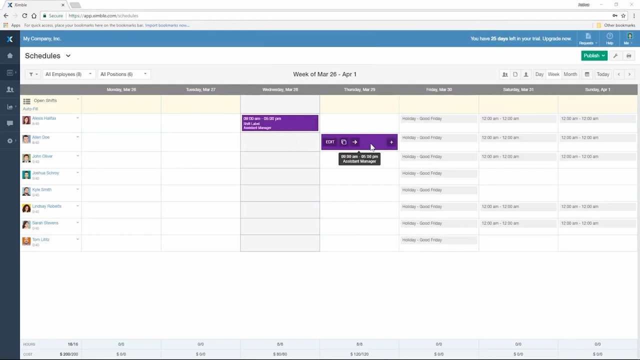 Zimbal. Let's start out our list with Zimbal, an easy-to-use employee scheduling and time-tracking tool where you can easily create, edit and assign shifts to employees. Apart from basic scheduling options, it allows employees to swap shifts or ask for time off directly from the app. 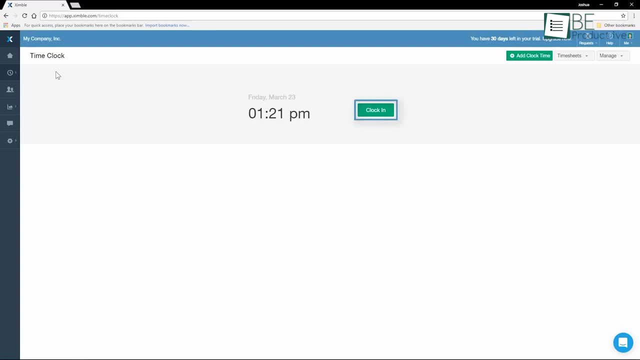 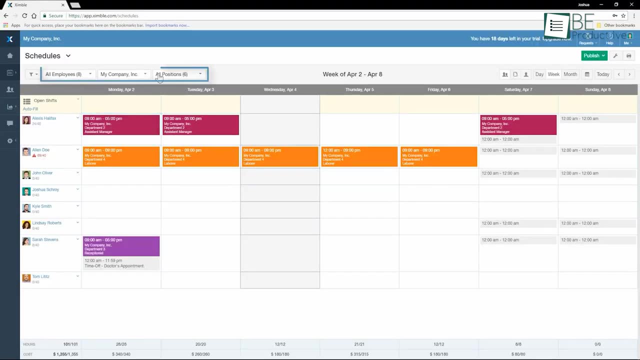 Employees can add different tasks in the time clock option and, using that, they can easily create and assign shifts to employees. In addition to that, you can review their shift activities and approve timestamps for payrolls. Moreover, it allows you to filter data based on location, time frame, position or department. 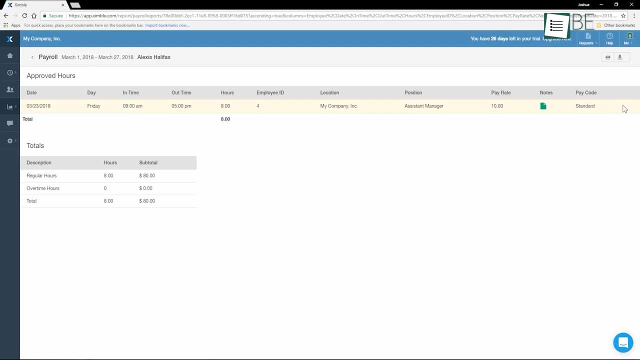 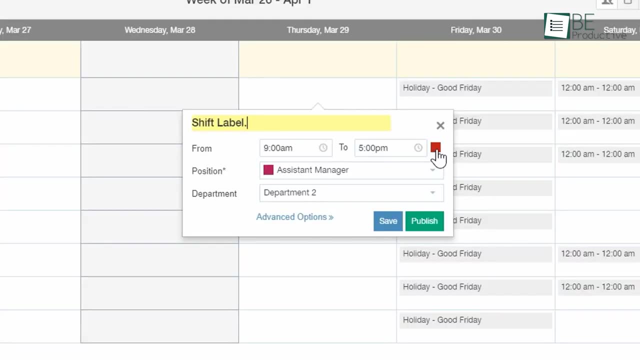 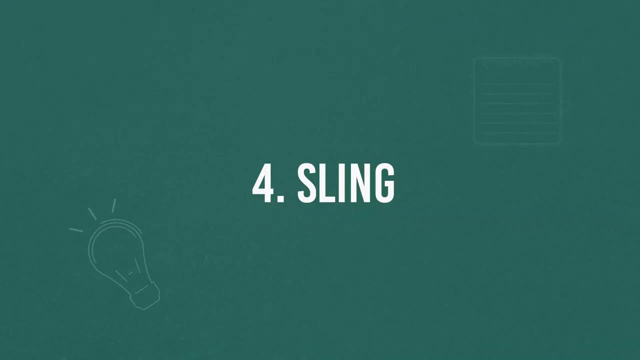 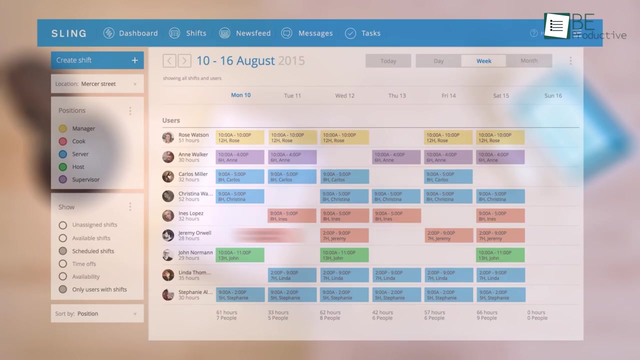 It offers automatic payroll management and allows you to stay connected with your employees all the time with Zimbal Chat. In addition to the 14-day free trial, it is totally customizable and allows you to choose between different paid plans. Sling- Next, we have Sling, an employee scheduling and communication app that allows you to 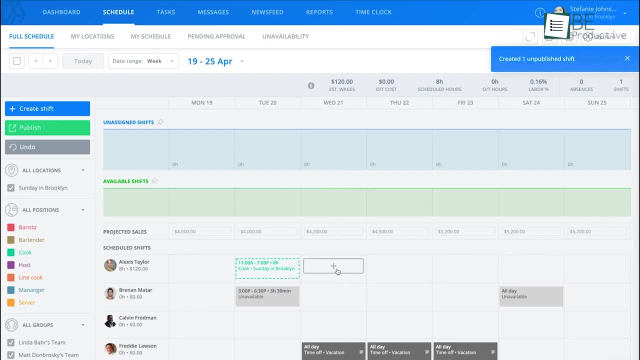 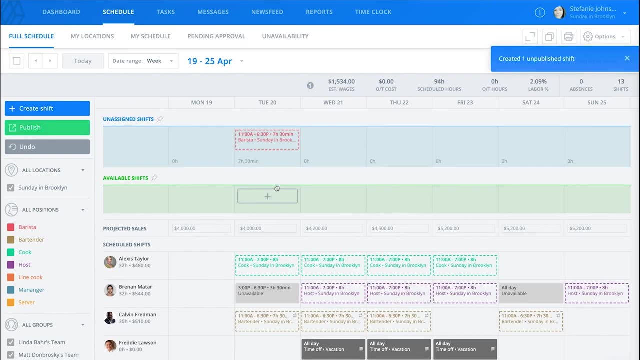 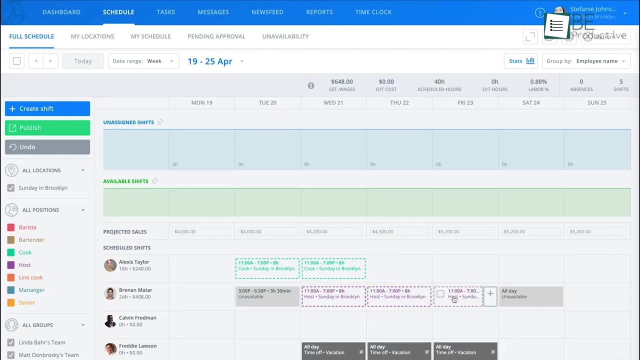 automate employee schedules, avoid overlapping shifts and communicate with employees. After completing the setup process, a schedule tab opens in front of you where you can create schedules, add shifts and also edit them if necessary. This app allows you to copy, drag or schedule recurring shifts more efficiently. Visibility of 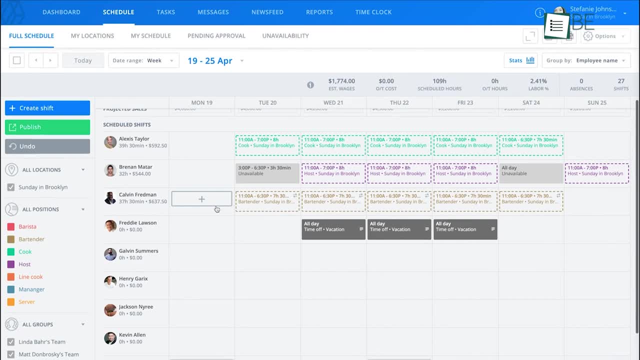 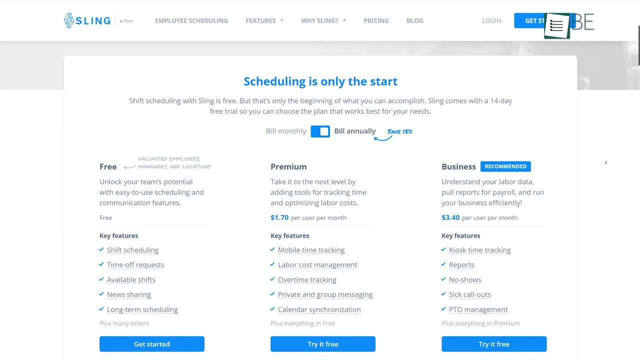 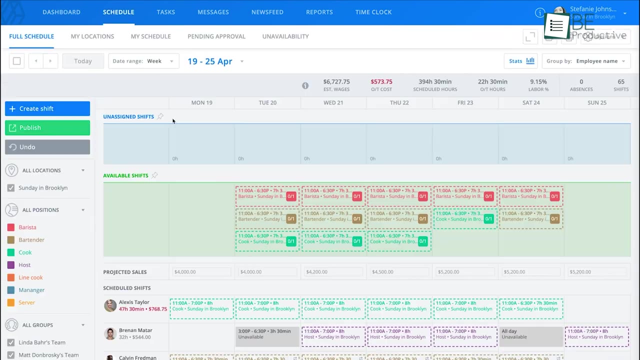 time off or unavailability of employees makes it easier to create shifts for employees. After the 14-day free trial, you can upgrade to a paid plan and get access to overtime alerts, labor cost management, mobile time tracking and so on. After scheduling the shifts, you need to publish it for the employees. 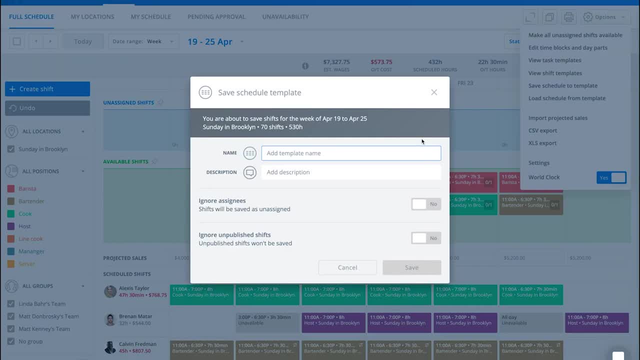 to get notified about their new shifts. Moreover, it allows you to save schedules as templates for future use. enfim: After scheduling the shifts, you need to publish them to get notified about their new shifts. Moreover, It allows you to save schedules as templates for future use. 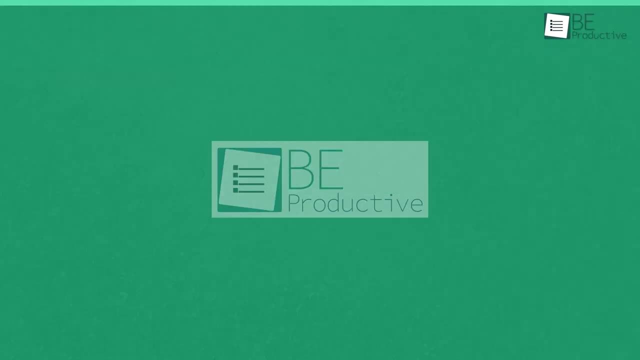 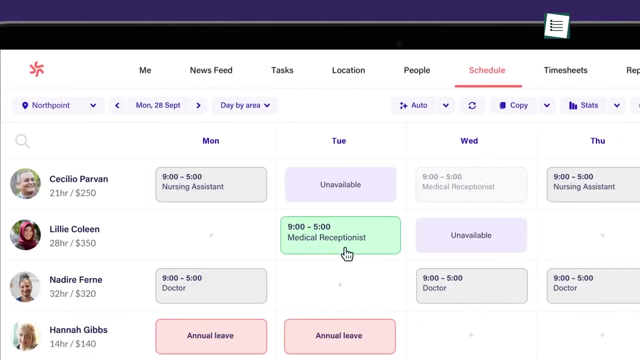 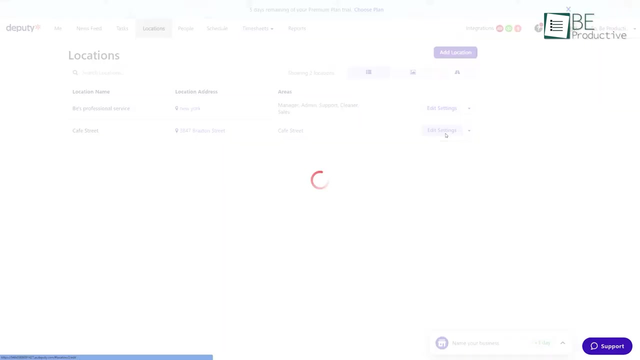 Coming up next, we have Deputy, a US-based tool for scheduling multiple employee roles in multiple locations. This comes with a 31-day free trial plan which enables a multi-location schedule and allows you to publish up to 100 shifts per month. 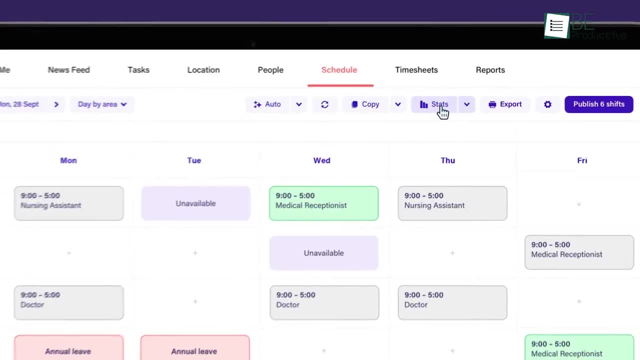 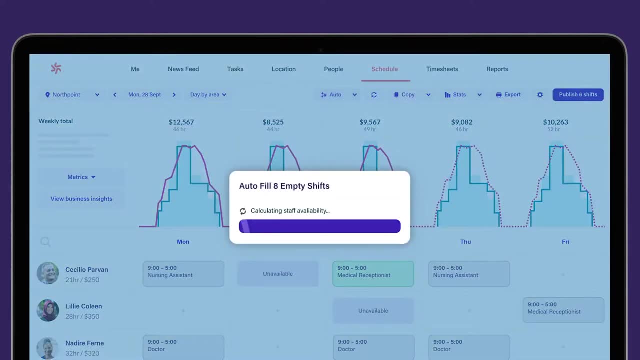 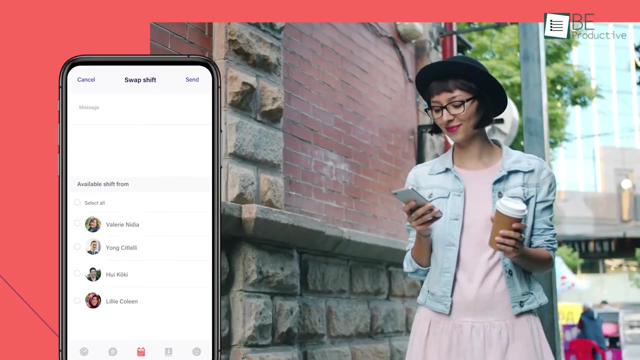 Deputy runs a five-point check ensuring training, stress profiles, leave, unavailability and overlapping whenever you create a shift. Moreover, it tracks employee qualifications to let you know whether that person is qualified for the assigned task or not, Like other software- finding a replacement, auto-filling an empty shelf and communicating. 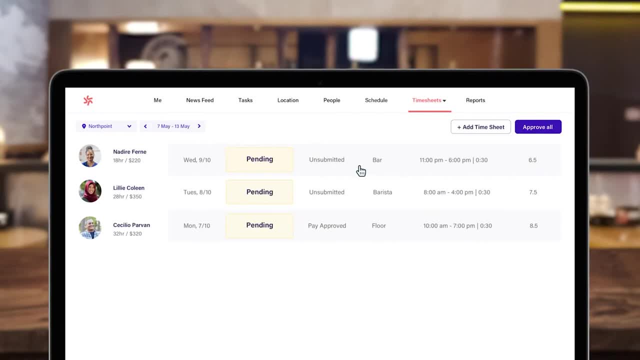 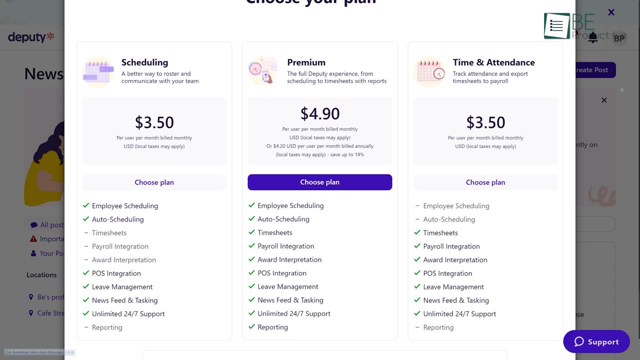 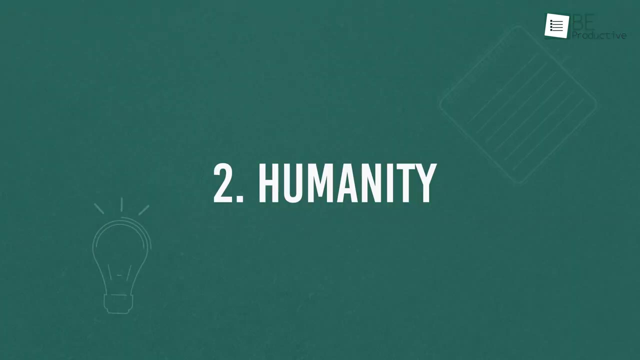 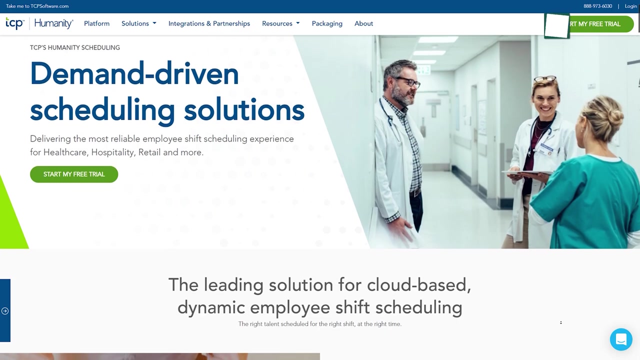 with employees are easier. Even though the free plan has limited features, you can upgrade to its affordable paid plan for separate time and attendance and scheduling options, Or you can choose a plan including complete solutions: Humanity, a cloud-based, fast and intuitive employee scheduling software that comes with. 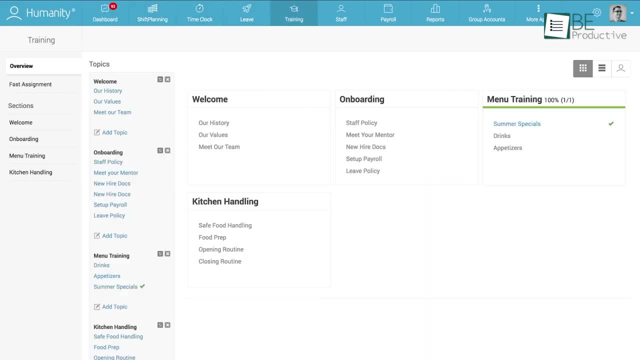 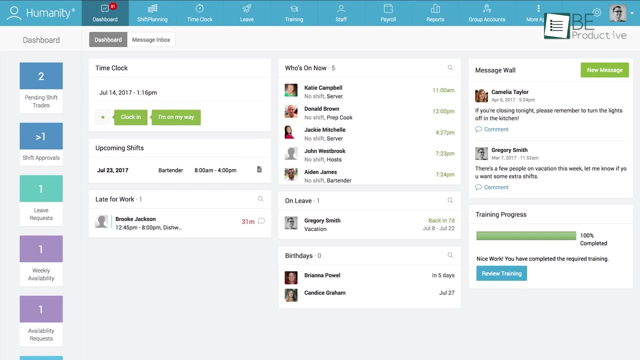 shift management, time clock, leave module, training module and payroll module for both managers and employees. One of its main attractions is the dashboard, where both managers and employees can access information like upcoming shifts, employees on-board, on-leave and on-go. 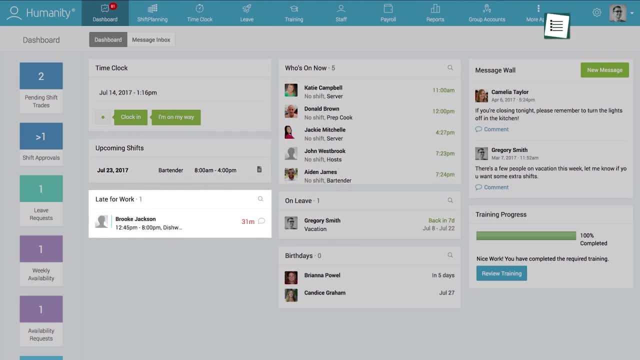 You can also plan a shift in a closed-off space. Humanity is an all-border system that allows you to get into the work space of both companies and employees, or late entry and also the birthdays of employees. in addition, the notification tiles help the user to go to the specific platforms. this comes with a 30-day free plan offering all the basic features. 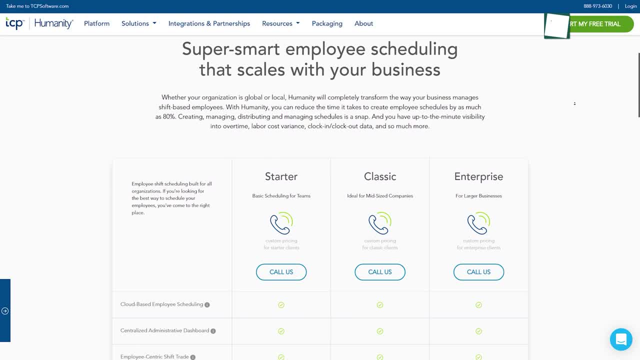 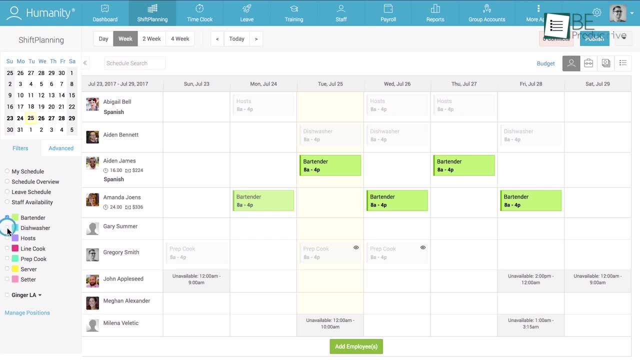 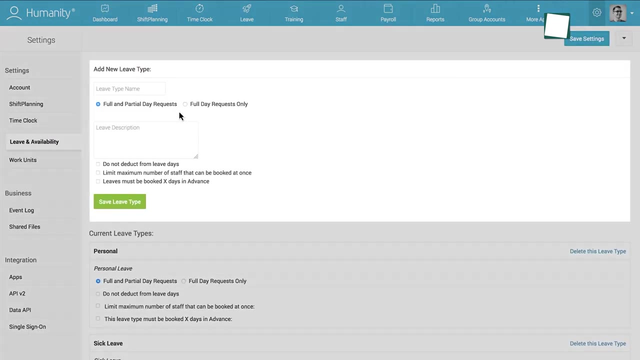 but you can customize paid plans according to your preference. the premium plan offers powerful features like advanced filtering options that provide managers with exact information to create error-free schedules. moreover, it offers skills and certifications, custom leave types and policies, and also allows managers to specify every detail of a shift.